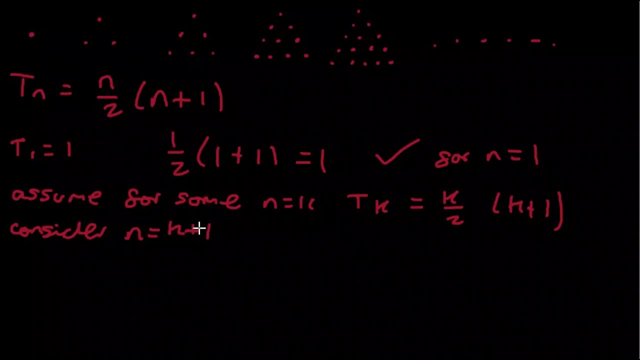 formula, the recipe, I guess, for all induction proofs. so we know that TK plus one is equal to TK plus one more term, and that term is K plus one. okay, so you see, because on the first term we add in one, the second term we add in two, on the third term we add in three. 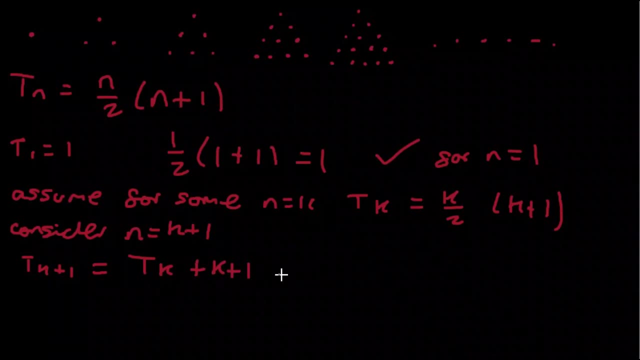 so plus K plus one, we've assumed that TK is equal to K over two, K plus one. and then we've got plus K plus one and we're going to factor out this K plus one, so that's K over two plus one. and then we're going to factor out this half, so that's equal to one half K plus one, K plus two. but we 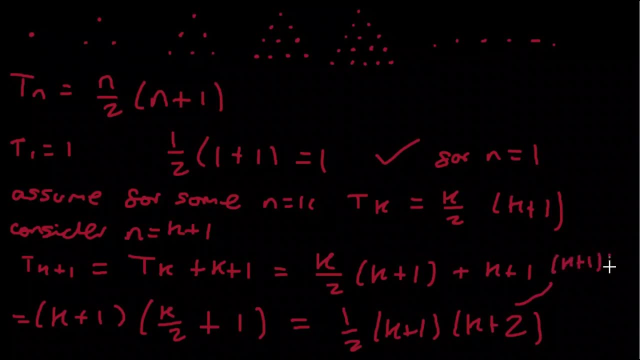 notice here: the K plus two is equal to K plus one, so that's equal to one half K plus one. K plus two is K plus one plus one. so this formula works for K plus one, given it works for K, and since we've shown it works for one. it therefore works for two, three, four, five, six, seven, eight, so on. and 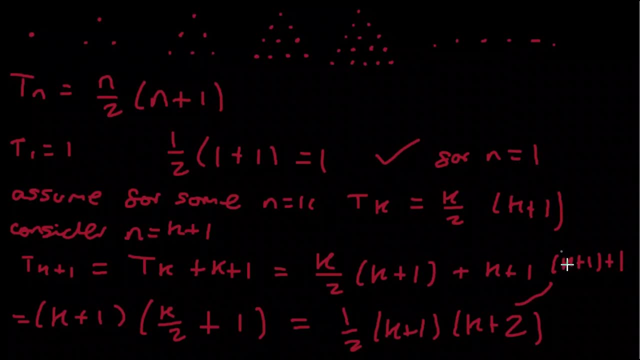 that we can continue that logic forever and therefore we've done our proof. you'd be required, on an exam or whatever, to write some sort of closing statement just to, just to justify the- it's just a couple of lines- and explain your steps as you go along. but I was having a much. 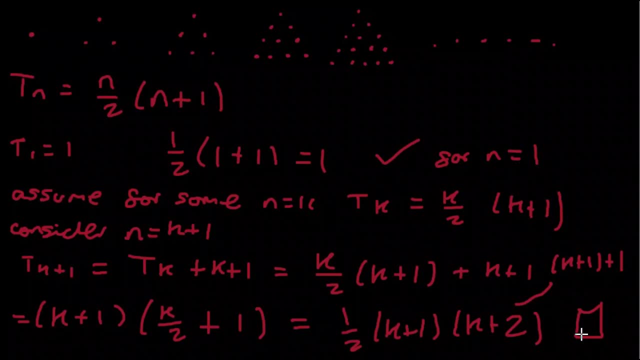 room here. so I just did the, did the math. a couple of questions on this method. so this step here, believe is, is obvious. but how do I know to factor out this K plus one? well, it just seems as a K plus one in each term seem like the the logical thing to do. you just try to rearrange this into the into. 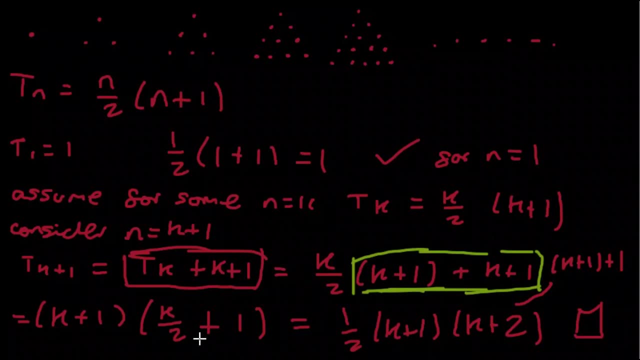 the correct form. and then, um, I noticed that once you take this half out, you're going to get a two here, which is what we want to get this result here okay, so, just a bit of trial and error, really, but the more you do with these, especially these types, because this is, despite being a question about